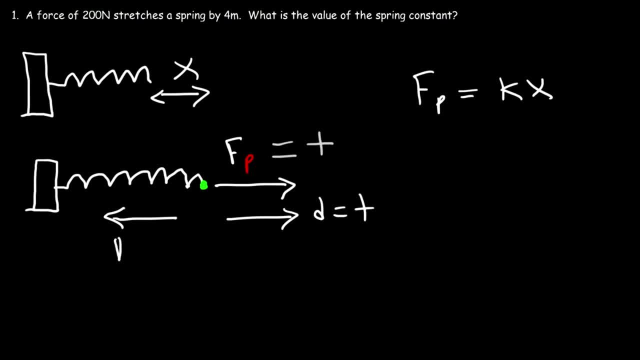 back to its original length. And that force, known as the restoring force, which you can call it fs or fr, and the restoring force is in the negative x direction. now, these two forces, they're equal in magnitude but opposite in direction, because once you apply a force, fp, the spring is at rest, it's not moving to the left or to. 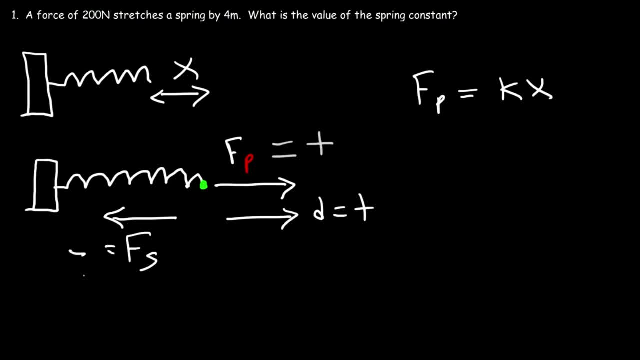 the right. once you let go, fs takes over and it's going to cause the spring to snap back to its original length. so because fs is a negative, we can say that the restoring force is negative kx, and this equation is associated with Hooke's law. so the magnitude of the restoring 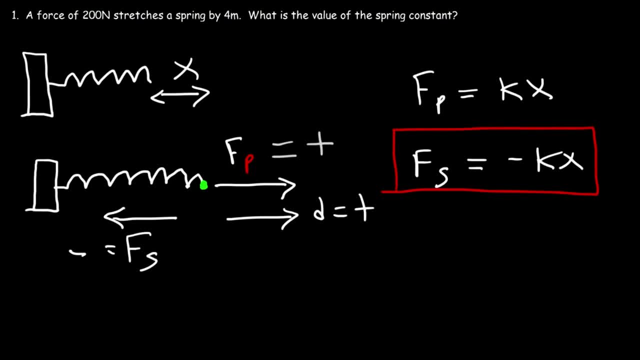 force is proportional to how much you stretch or compress the spring from its natural length. so now that you've received a basic introduction into Hooke's law, let's go ahead and focus on finishing this problem. so number one: a force of 200 newtons stretches the spring. 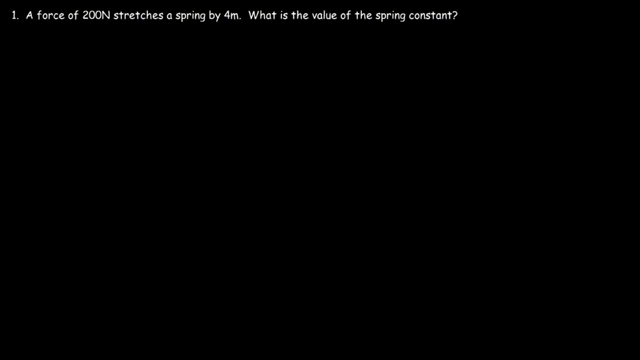 by four meters, what is the value of the spring constant? so if the force that we use to stretch it, which is fp, is equal to kx, then the spring constant k is simply the ratio of the force and the distance that you stretch the spring. so we have a force of 200 newtons and it stretches the 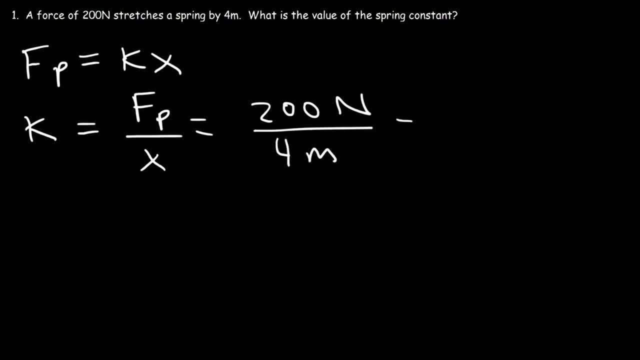 spring by a distance of four meters. so 200 divided by 4 is 50.. and we see the spring constant has a unit newtons per meter, so it's 50 newtons per meter. so what this means is that in order to stretch the spring by a distance of one meter, a force of 50 newtons is required. 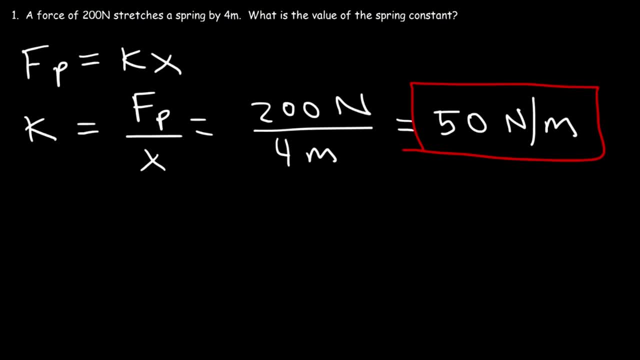 in order to stretch it by two meters, you need a force of a hundred newtons. do so, And so the spring constant. it tells you how much force you need to stretch a spring by one meter. So let's say, for example, if the spring constant was 300 newtons per meter. 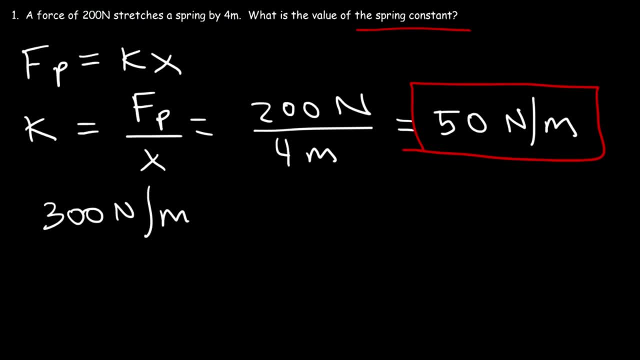 That means a force of 300 newtons is required to stretch a spring by one meter. Now, looking at these two spring constants, which one is more stiff? The spring, that's 300 newtons per meter or 50 newtons per meter. 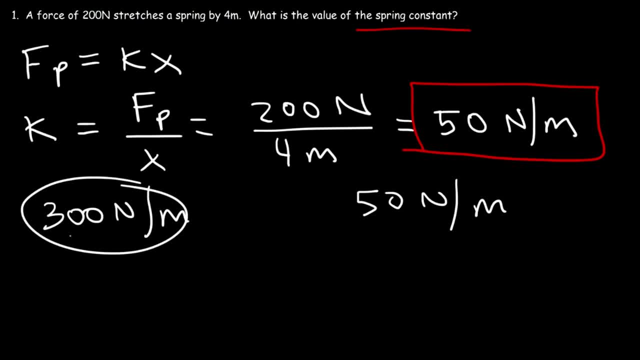 This spring is going to be more stiff. It's going to be hard to stretch or compress the spring because it has a higher spring constant. This spring is going to be loose. It's one of those light springs that you can easily pull apart. So as k increases, as the spring constant. 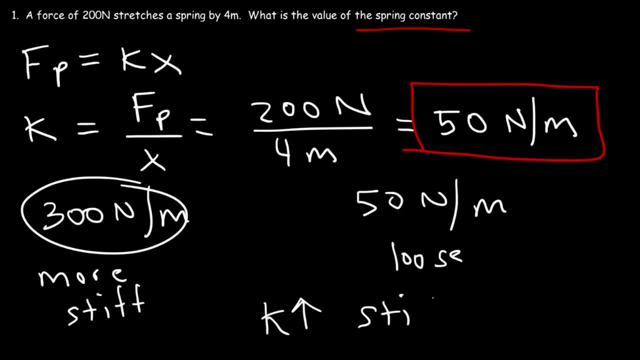 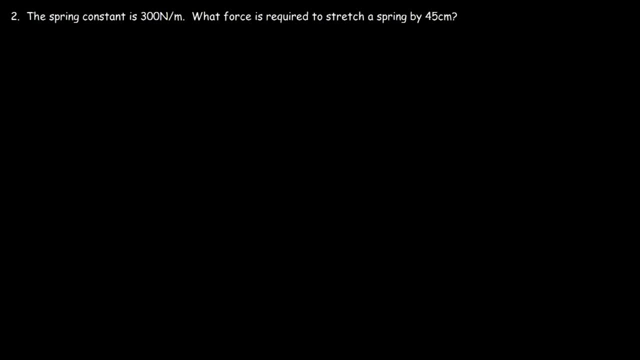 increases in value, the stiffness of the spring increases as well. Let's move on to number two. The spring constant is 300 newtons per meter. What force is required to stretch a spring by 45 centimeters? So let's use this equation: Fp is equal to kx, So our goal is to find Fp. 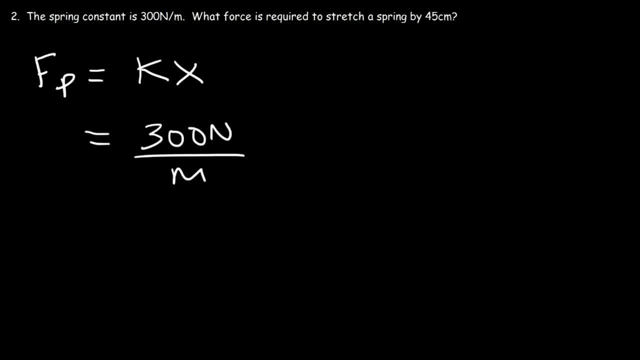 K is 300 newtons per meter. Now we don't have x in meters, We have it in centimeters, So we need to convert that to meters. In order to convert centimeters to meters, you need to divide by 100.. One meter is 100 centimeters, And so these units will. 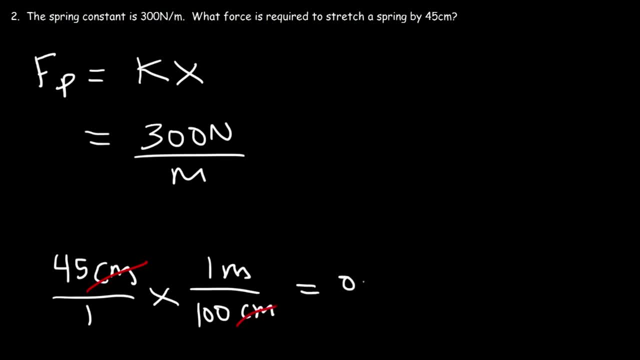 cancel. 45 divided by 100 is 0.45 meters. So if we multiply the spring constant by 0.45 meters, we can see that this is going to give us the unit newtons, which is the unit of force. 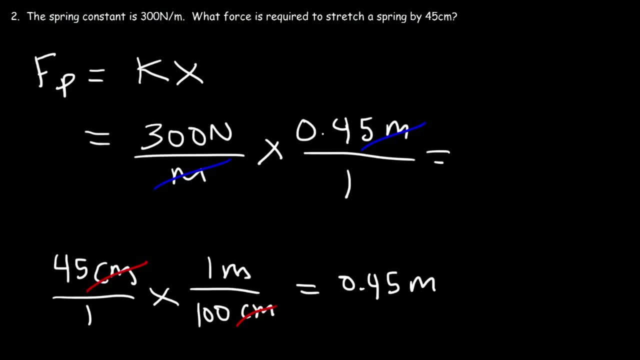 So it's 300. times 0.45, and so that's going to be 135 newtons. So that's the force that's required to stretch the spring by 45 centimeters. Keep in mind, if the spring constant is 300 newtons per. 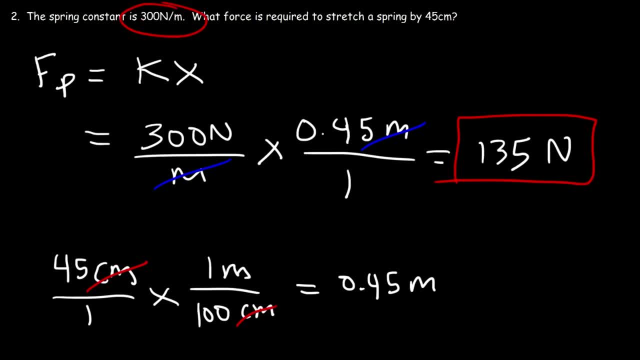 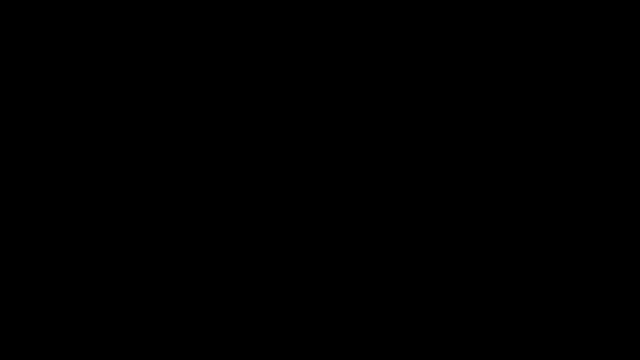 meter. in order to stretch it by one meter, it requires a force of 300 newtons. So thus to stretch it by half a meter would be 150 newtons. So 0.45 meters, which is just under a half, would make sense that it's 135 newtons. It's always good to take a mental check of your answers, So let's. 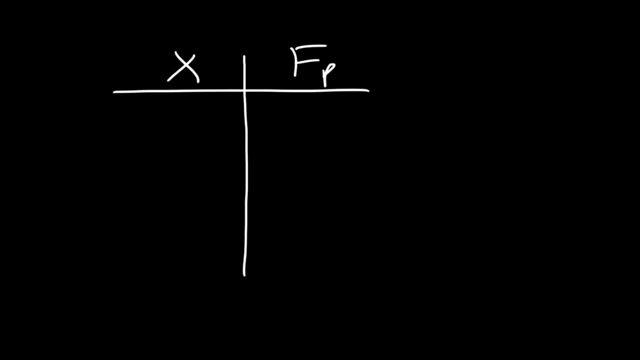 make a table between X and the force applied. So the spring constant was 300 newtons per meter. So that means at a distance of one meter a force of 300 newtons is required. So if we divide the distance by half a meter we get a force of 300 newtons per meter. So that means at a distance 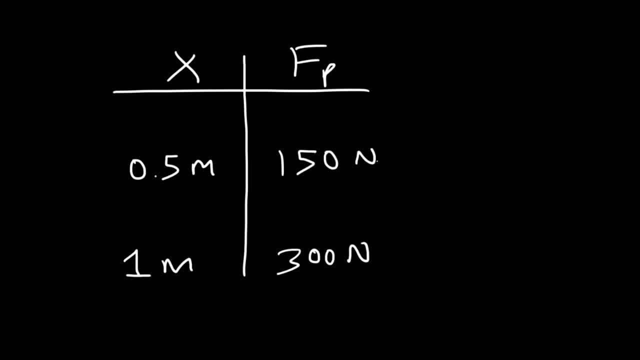 by two. we should divide the force by two. So therefore our answer at 0.45 meters is 135, which makes sense. So this is less than 0.5 and this is less than 150.. So always check to see if your. 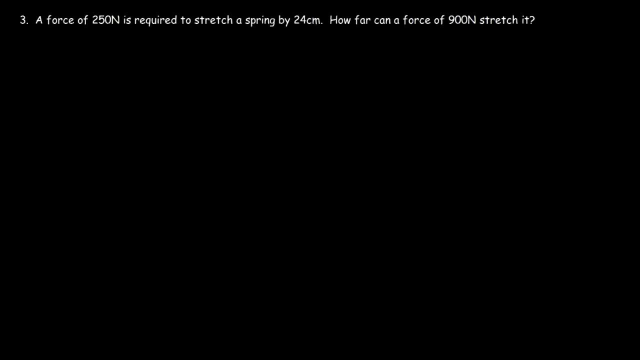 answer is reasonable. Does it make sense? Now let's move on to number three. A force of 250 newtons is required to stretch a spring by 24 centimeters. How far can a force of 900 newtons stretch it? So we're given a force and a distance and we're 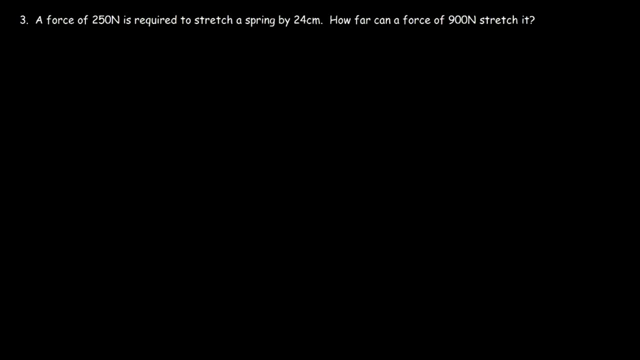 given another force and we're trying to find another distance. You could find a spring constant K or you could come up with another equation to do this. So I'm going to show you two ways of getting the answer. The first is to calculate the spring constant K. It's going to be the force divided by 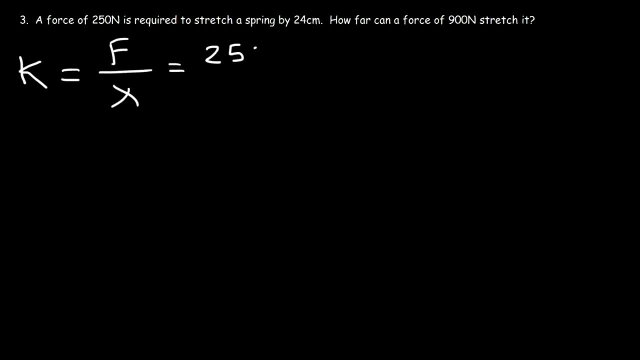 the distance. So a force of 250 newtons is required to stretch a spring by 24 centimeters. So a force of 250 newtons is required to stretch it by 24 centimeters, which is 0.24 meters if you divide it. 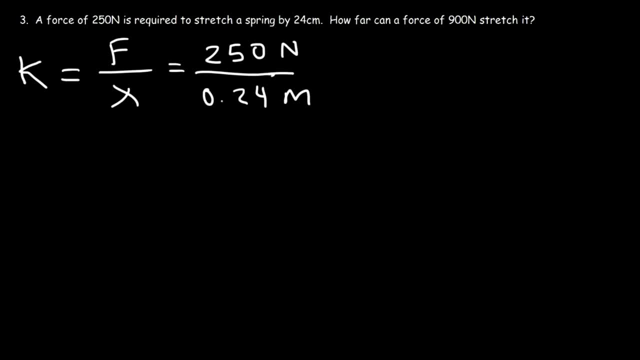 by 100.. So 250 divided by 0.24 will give us a spring constant of 1041.6 repeated. Now to find out how far it's going to stretch, we need to calculate the value of X, and X is F divided by K. So we have a new force of 900 and we're going to divide it by 1041.6. 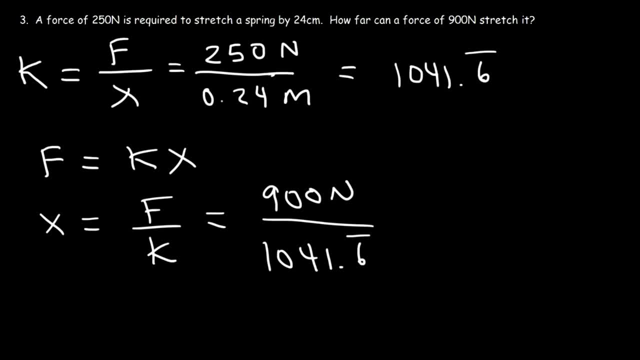 repeated. So this is going to be about 0.864 meters, which in centimeters is 86.4 centimeters if you multiply it by 100.. So that's one way in which you can get the answer. Now let me show you another way. 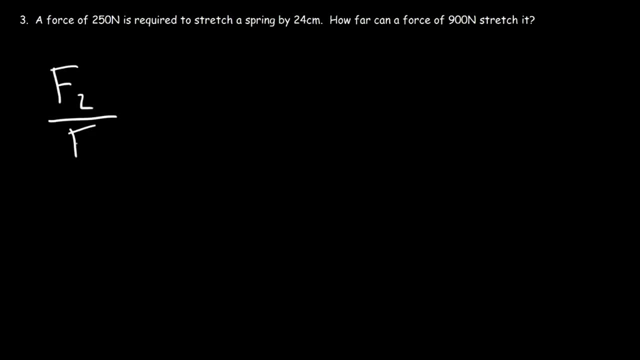 Let's take the second force and let's divide it by the first force. The second force is K times the second distance, and the first force is K times the first distance. So because K is the same, we can cancel it. So therefore, the ratio of the 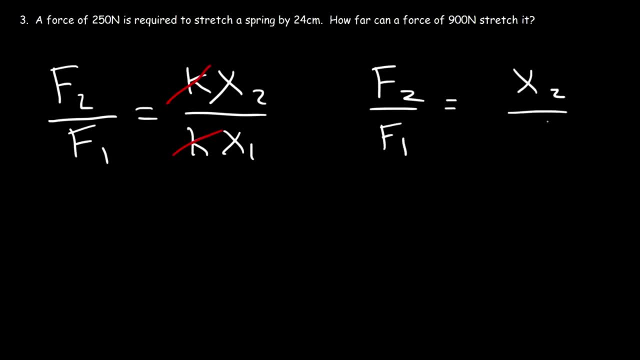 forces is equal to the ratio of the displacements in X, and it makes sense because X and F are proportional to each other. So we're going to call this F1, and this is going to be X1, and this is F2 and we're looking for X2.. 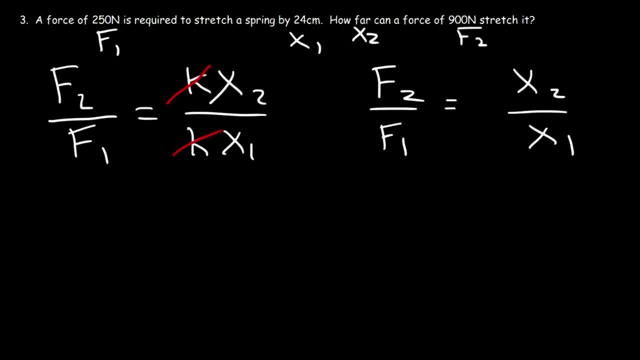 Now the unit centimeters will cancel, so it doesn't matter if you use meters or centimeters when dealing with ratios. the ratio will still be the same. So let's replace F2 with 900 newtons and F1 with K with 250 Newtons. Our goal is to calculate X2, and X1 is 24 centimeters, So let's cross-multiply. 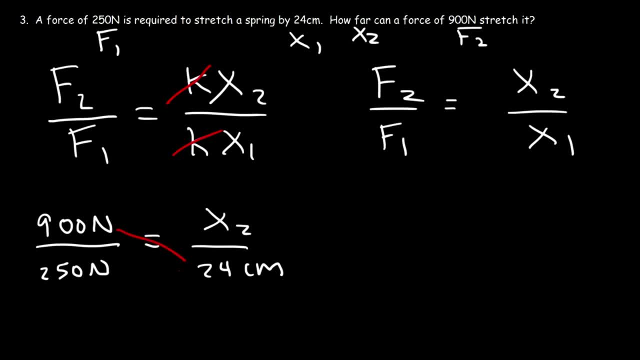 So first we have 900 times 24,, so that's 21,600 with the units Newtons times centimeters, and that's equal to 250 Newtons times X2.. Now, in order to get X2, we've got to divide. 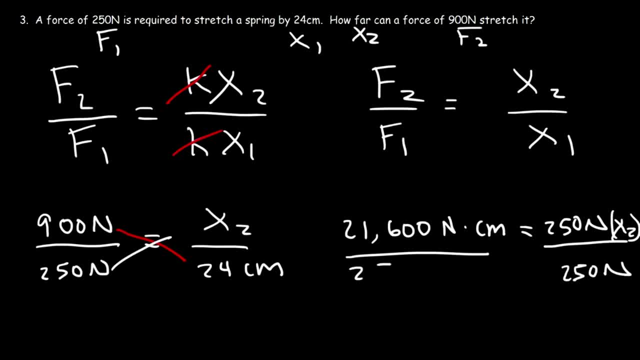 both sides by 250 Newtons. On the right side, these two will cancel, giving us X2.. On the left side, notice that the units Newtons will cancel, leaving behind centimeters, which is going to be the unit for X2.. 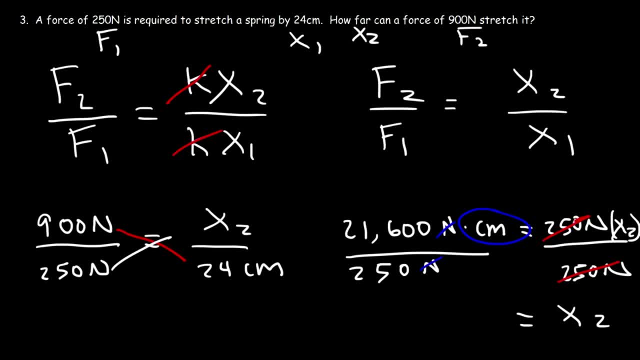 So it's 21.. 21,600 divided by 250, and so you're going to get 86.4 centimeters. So you have two ways in which you can get the same answer. Consider this problem: How much work is required to? 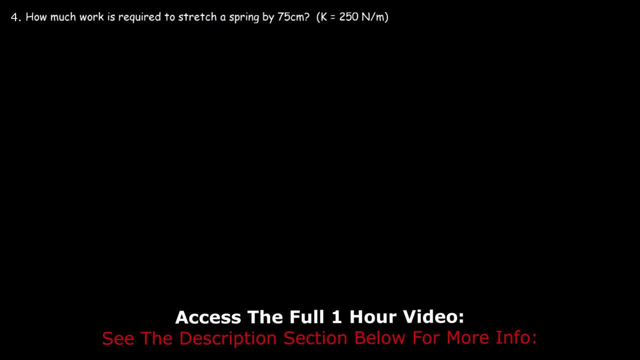 stretch a spring by 75 centimeters And we're given the spring constant. So let's draw a spring Now. the force, The force that's required to stretch a spring above its natural length- let's say this is the natural length of the spring- is: 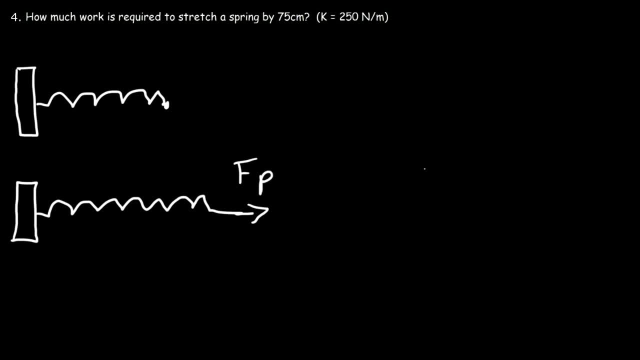 We're going to call it Fp. Now, Fp is equal to Kx. Now, once you stretch it and you stop stretching it, you still need to apply a force to hold its position. Now, if it's at rest, that means that there's an equal and opposite force that wants to. 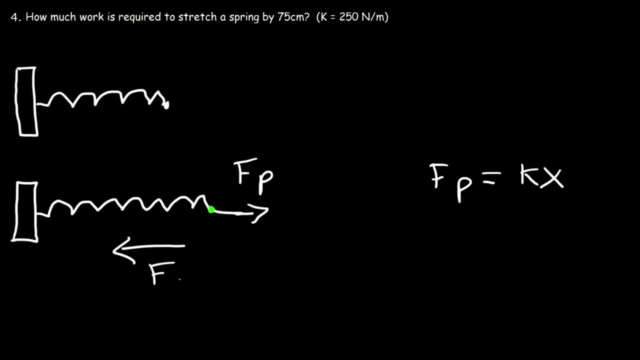 snap back, the spring back to its natural length, And that is the restoring force. Now, this force is positive, It's going in the positive X direction And this force is negative. So according to Hooke's Law, the restoring force is negative Kx. But we're. 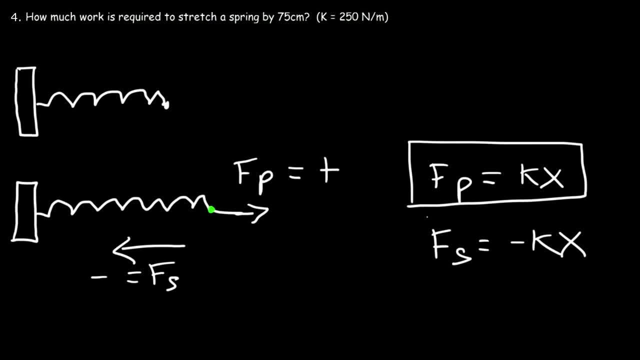 going to focus on this force. How much work is done by this force in order to stretch the spring by a displacement X? X is the distance between It's, between the natural length of the spring and its current length. So it's how much it. 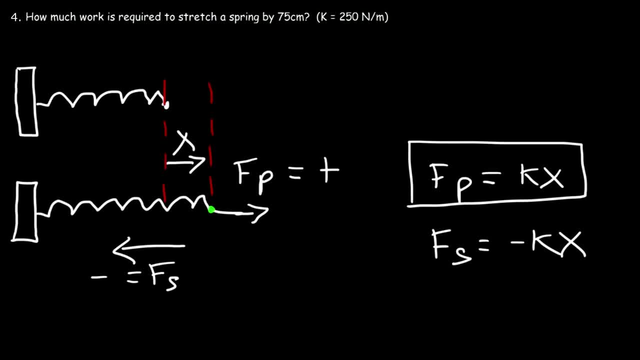 stretches or compresses. by Now work is equal to force times displacement. So the displacement is X, So work is equal to Fx. Now, F is not a constant value. F depends on X, F is a function of X. So if we were to make a graph between force and displacement, it would look something. 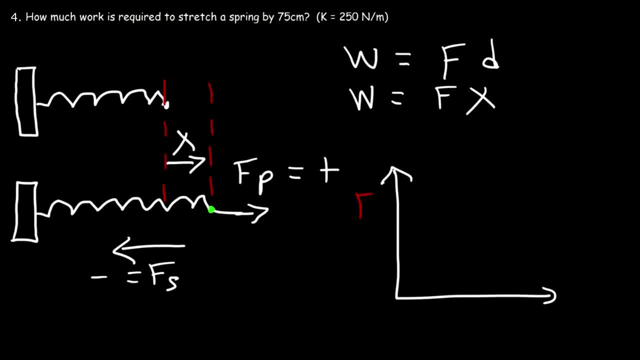 like this. Now, F is not a constant value, but it's a function of X. It's equal to Kx, So what we have is a linear equation where the slope is K, So this is going to be a straight line that looks like this: 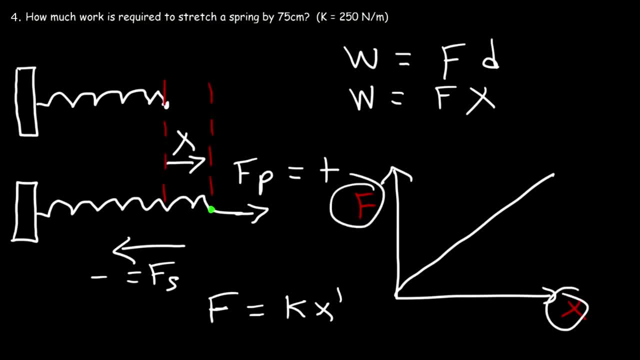 Now, whenever you have a force displacement graph- Yes, For inheritance. Now, if you remember you looked at this- annoys. There is no normal. We know that work is force times displacement, but for such a graph the work is equal to the area under the curve. 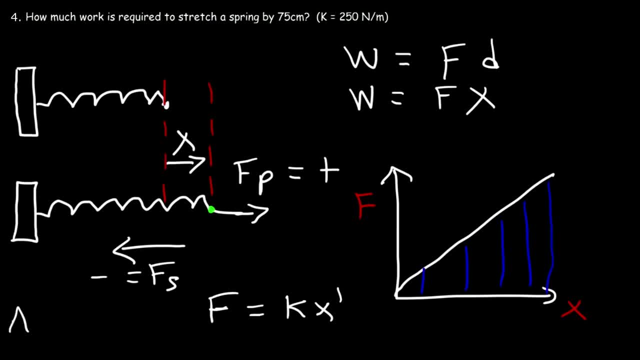 So what is the area of the triangle? The area of a triangle is 1 half base times height. In this example, the base of the triangle is equal to x and the height of the triangle is equal to f. So therefore, the area is 1 half f times x, where f is the maximum force value at a distance x. 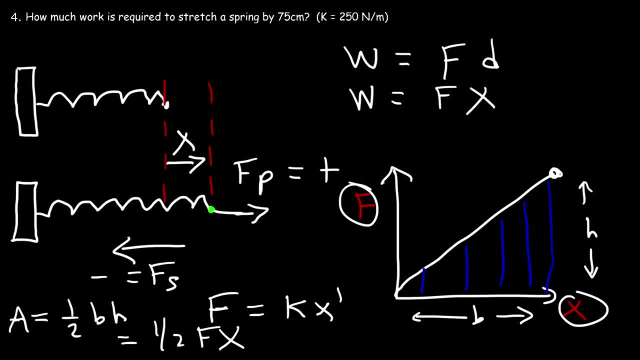 So this equation holds true if the force is constant. So if you had a graph where this is f and this is x and the force was constant, the area will be the area of the rectangle which is left times width. That will be simply f times x. 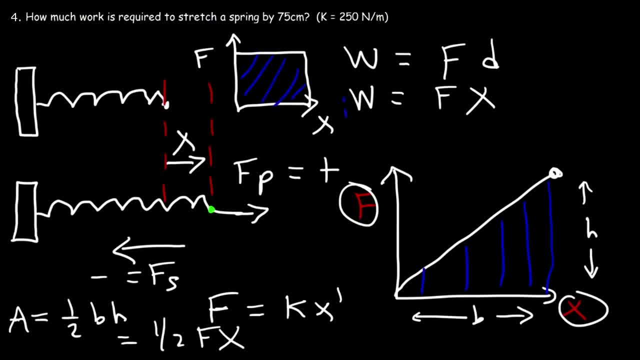 There won't be a half, That's if the force is constant. Now what we have is a variable force that increases according to the displacement or how much you stretch it. So therefore, the work done by that variable force is the area under the curve, which is 1 half f times x. 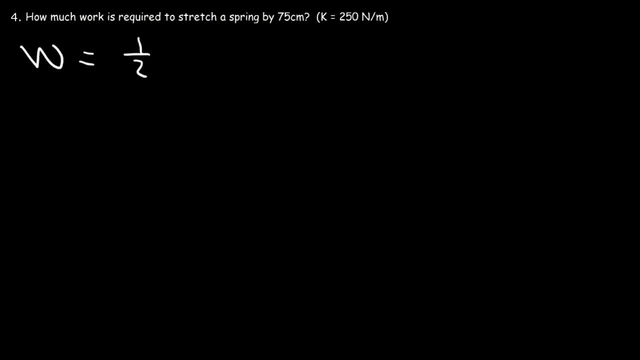 So the work required to stretch a spring is 1 half times the force. The variable force is 1 half f times x, The maximum force times x, And based on Hooke's Law we know that f is equal to kx. 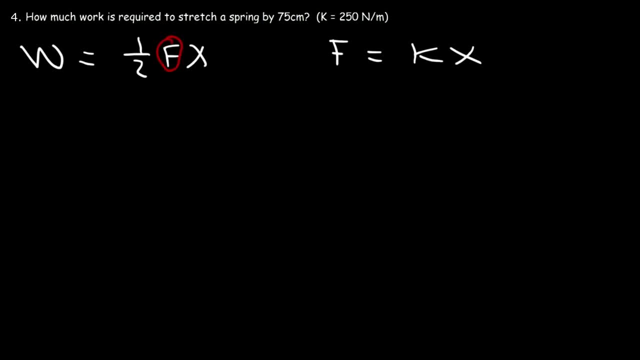 So what I'm going to do is replace f with kx And keep in mind this x is really delta x. So this is going to be k delta x and this is supposed to be delta x, because it's really the change in the position. 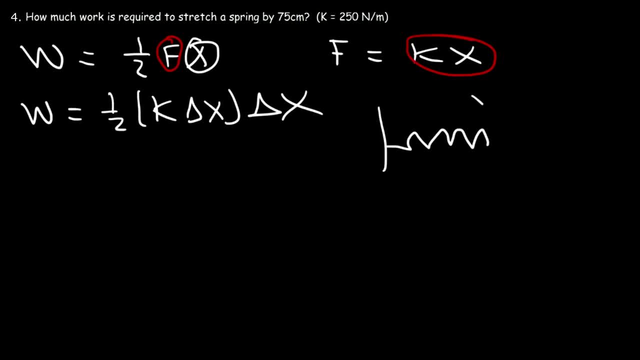 So let's say, if this is the natural length, So let's say, if this is the natural length of the spring, it's at position xa and you stretch it to a new position, xb. This is the difference between xb and xa. 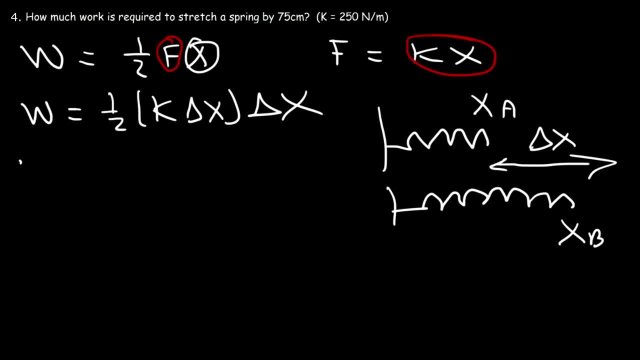 So technically it's delta x. So therefore, the work required to stretch a spring is going to be 1 half k times delta x squared. So this is the equation that you want to use. So k is 250 newtons per meter and we want to stretch a spring by 75 centimeters. 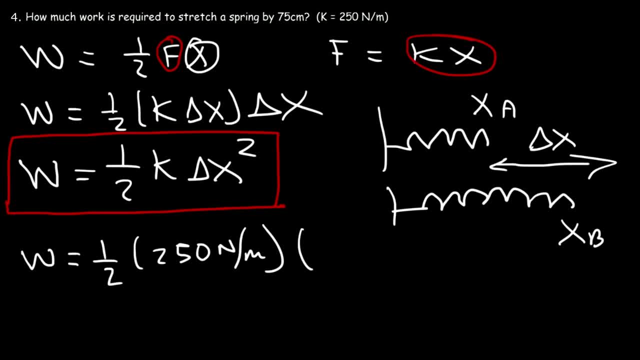 However, we need to convert that to meters. To convert centimeters to meters, divide by 100. So this is going to be 0.75 meters squared. So it's 0.75 squared times 250 times 0.5.. 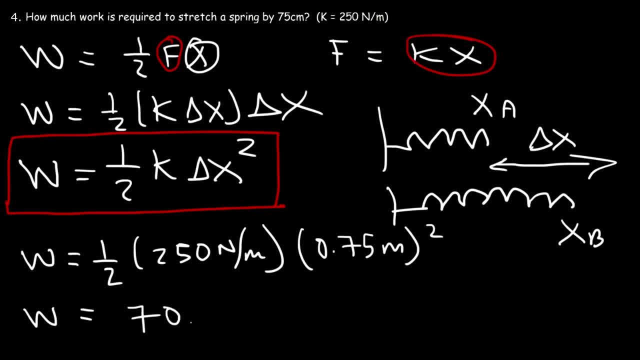 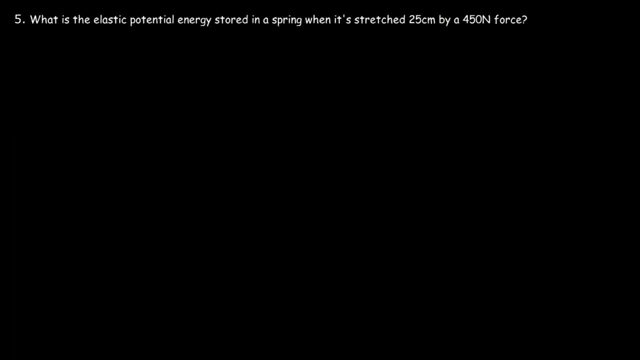 So, therefore, the work required is 70.3 joules of energy. Now, what is the elastic potential energy stored in a spring when it is stretched 25 centimeters by a 450 newton force? So let's come up with the equation to calculate the elastic potential energy. first, 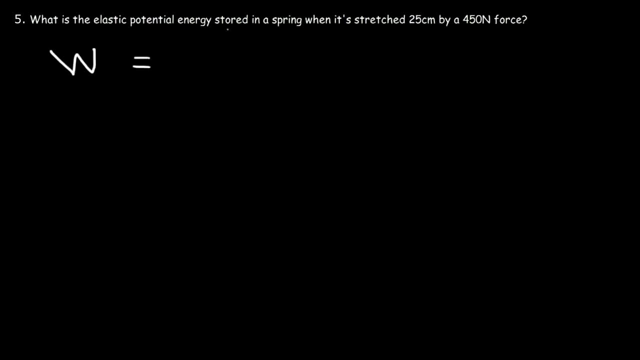 So we said that the work required to stretch a spring by the applied force is 1 half k delta x squared. Now, the work done by such a force is equal to the change in the potential energy if the acceleration is 0.. Which it is. 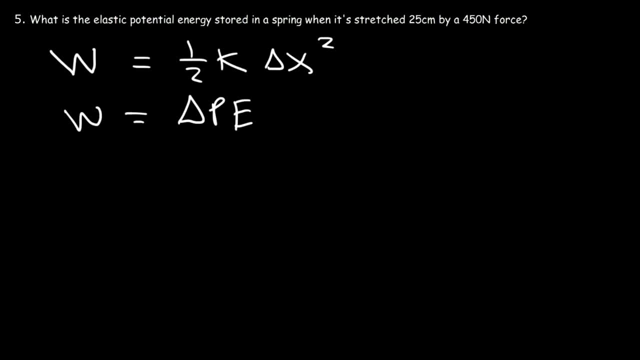 The applied force and the restored force. they're equal to each other. So work is equal to the final potential energy minus the initial potential energy. Now some textbooks may describe the elastic potential energy as US Capital U can be described as potential energy. 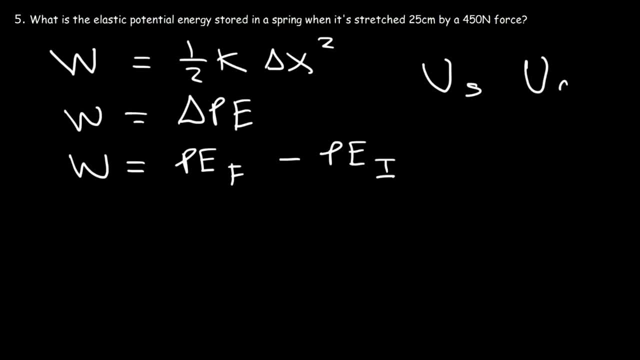 So if you see US, that's elastic potential energy, UG, gravitational potential energy, So just keep that in mind. I like to use PE because PE potential energy, it makes sense. So what I'm going to do is replace the W with this expression. 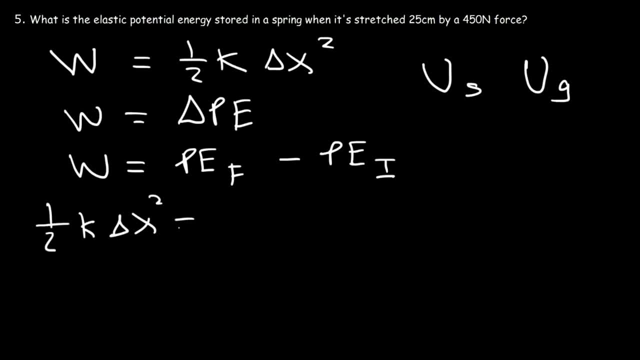 So 1 half k delta x squared is equal to the stuff that we have on the right And delta x is basically the final position minus initial position. So we have 1 half k x final squared minus x initial squared. So 1 half k x final squared minus 1 half k x initial squared. 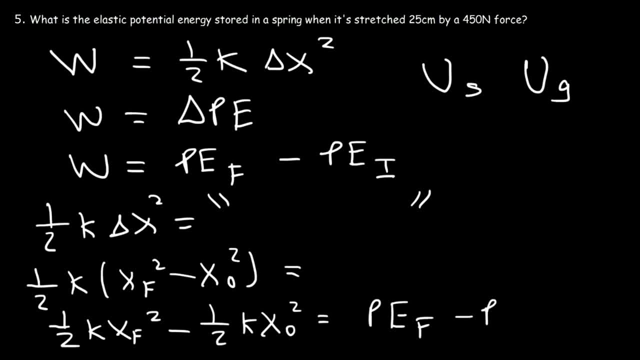 is equal to the final potential energy minus the initial potential energy. So what does this all mean? Well, we can see that this is equal to the final potential energy And this is equal to initial potential energy. Therefore, the elastic potential energy in general is simply 1 half k x squared. 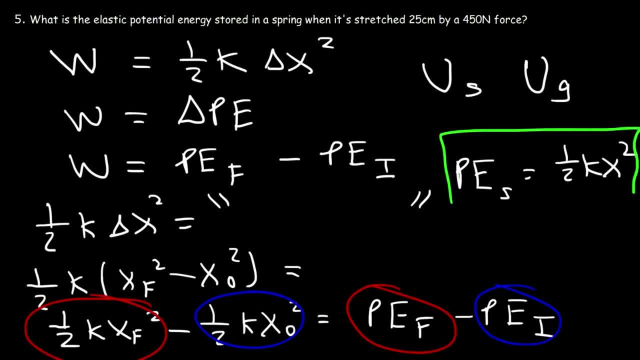 So notice the difference between this equation and this equation. So what do you notice? The work depends on the change in position, Whereas the potential energy. it depends on x, And x by itself. it has to be relative to the natural length of the spring. 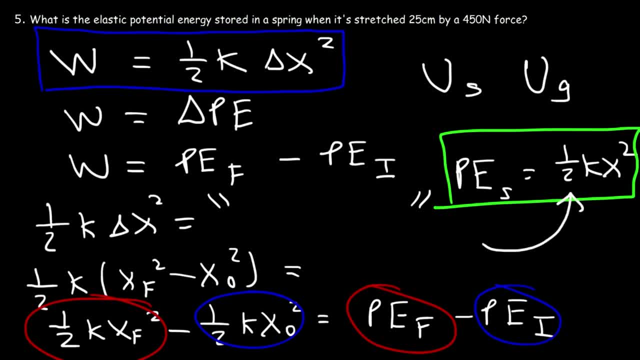 So the potential energy is based on the relative length between where you are and the natural length of the spring. The work required doesn't have to be associated with the natural length of the spring. It's simply the energy required to move it from position A to position B. 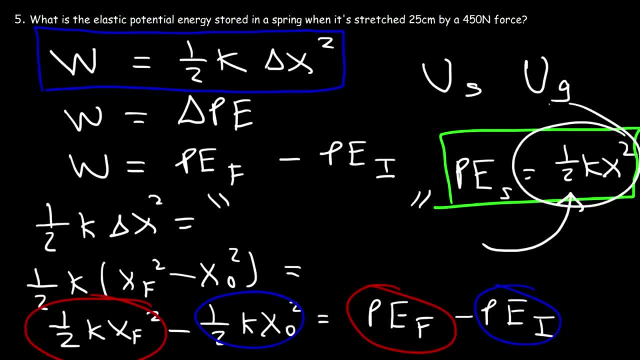 For this equation, position A has to be the natural length of the spring, But for this one, position A or B does not have to be the natural length of the spring. So keep that in mind. When I mean natural length, you can also describe it as the natural position of the spring. 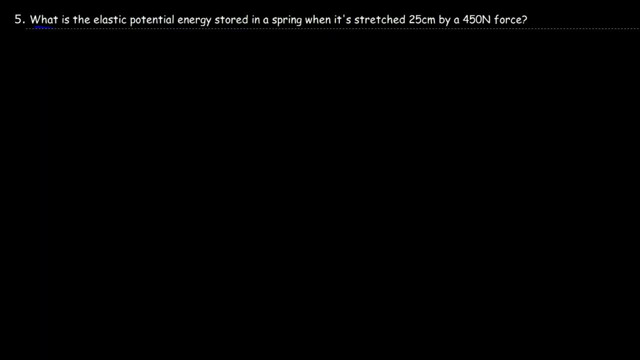 Which is usually defined as x equals 0.. So let's focus on this. What is the elastic potential energy stored in the spring? So we're given x and we're given the force F, So we know that the elastic potential energy is one half k, x squared. 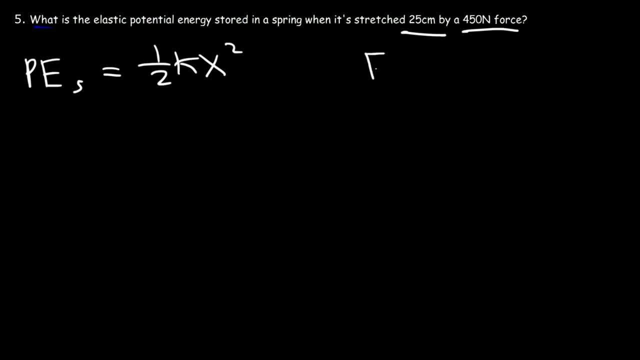 The only thing we're missing is k, So we could find k using this equation: F equals k, x, So k is the ratio between the force and the displacement. In this case, k equals force F, So we give the force at constant into k. 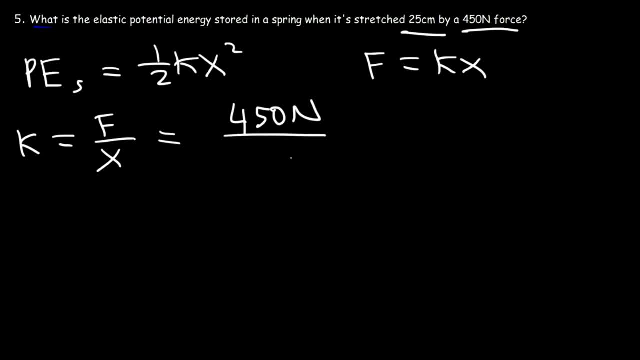 We ask for the force and distance from a spring And according to this equation, f equals, u increases, the stiffness of the spring increases. so just to stretch the spring by distance of one meter requires a force of 1800. that's what the spring. 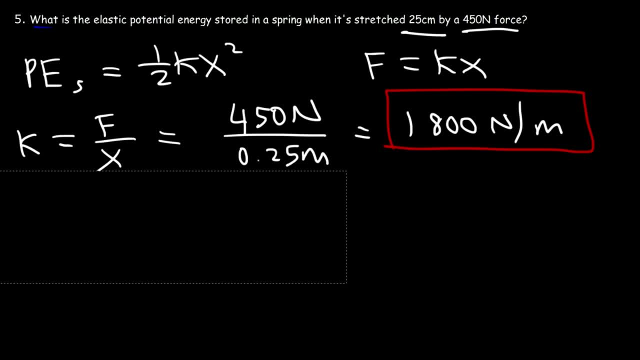 constant tells us. so now that we have K, let's calculate the potential energy. so it's one half times K times x squared, where X is 0.25 meters. so point 25 squared times 1800 times 0.5, that's equal to 56 point 25 joules, and so 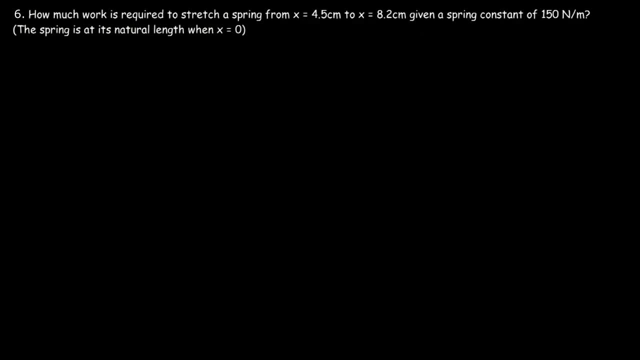 that's the answer. how much work is required to stretch a spring from 4.5 centimeters to 8 point two centimeters, given a spring constant of 150 newtons per meter? so let me give you a visual first of what we have here. so let's say this is the 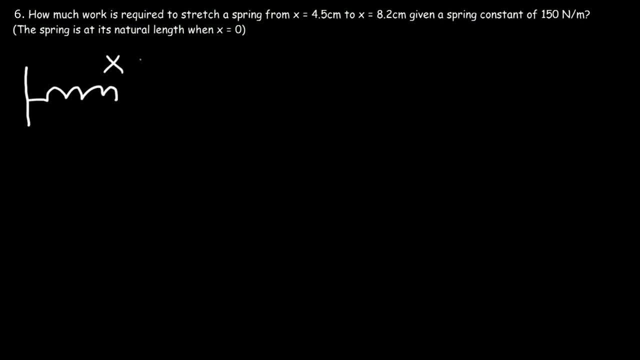 spring at its natural length. so at this point X is equal to zero. now the spring is currently stretched to this position- let's call it XA- that's when X is equal to four point five, and we need to calculate how much work is required to stretch it further to position B, where X is eight point two centimeters. so how? 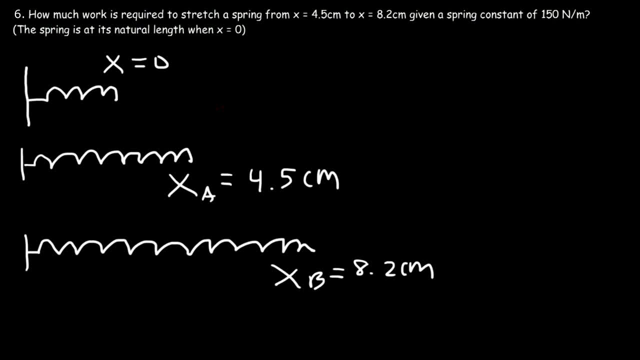 can we find the work required to go from position a to position B? go ahead and try that problem. the equation that you need is this one: one-half kx. I mean k times Delta x squared. now I need to be careful, because there's something you don't want to get. 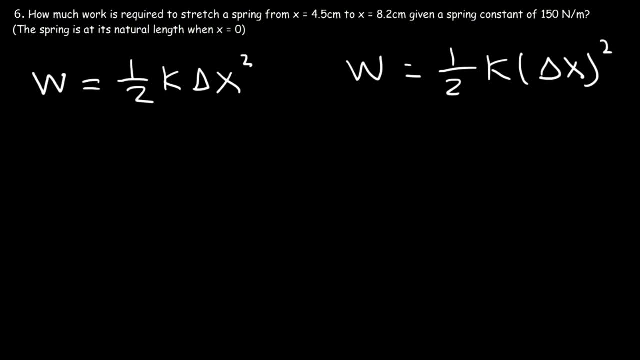 mixed up with. when I wrote this expression, I meant that Delta x squared is equal to one-half k times x final squared minus x initial squared. so not like this, not one-half kx final minus x initial squared. if you do it this way, you'll get the wrong answer. so 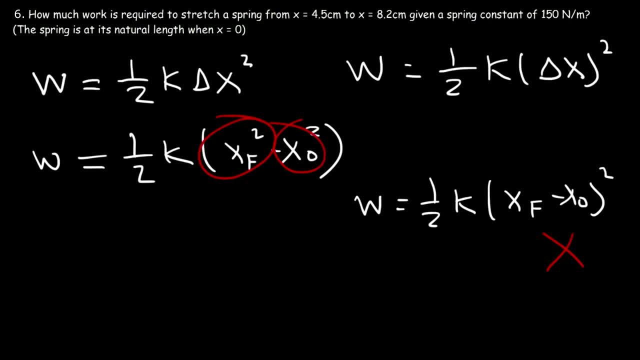 it's the difference of the squares of x, not the square difference of the x values, if that makes sense. so this is the right way to calculate it, because then work is equal to the change in potential energy. so if you do it this way, you're not going to get the right answer. I just want to highlight. 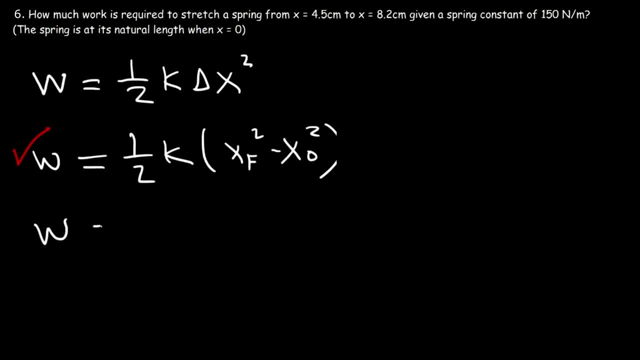 that point. so it's going to be one-half times the spring constant, which is 150 times the square of the final position, which we need to be in meters. so that's going to be point zero eight two meters squared, minus the square of the initial position, which is point zero four five meter squared. so go ahead and type this: 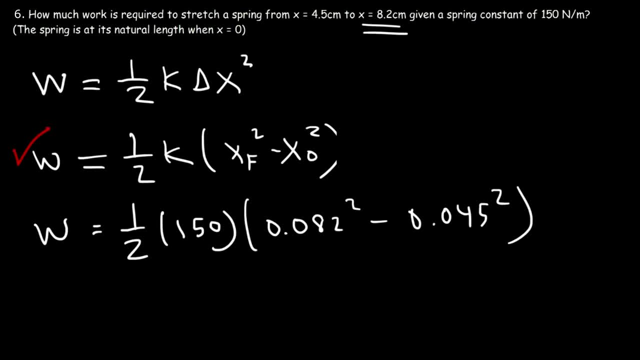 in exactly the way you see it. so you should get point three, five, two jewels for the work required to stretch it from position a to position b. now, for those of you who might be interested in, you may want another way to verify this answer: calculate the potential energy. 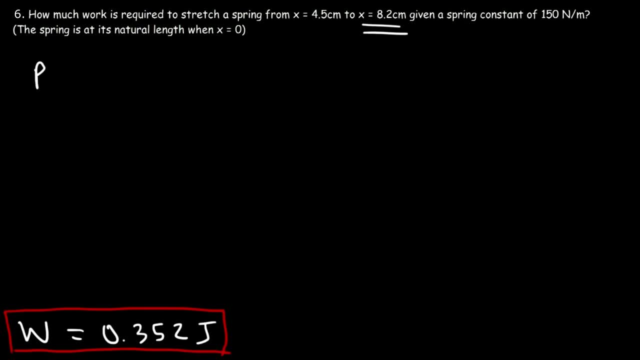 at point a and b. so the potential energy at point a is going to be one-half kx squared where x is at position a. so it's one-half times 150 times point zero, four five meters squared. so at position a the elastic potential energy is 0.1519 joules. now let's 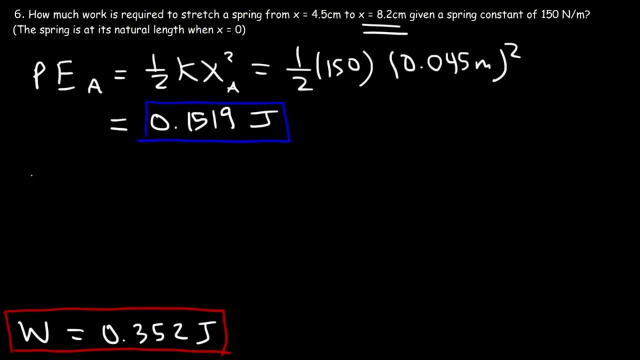 calculate the elastic potential energy at position b. so it's one-half kxb squared, so that's one-half times 150 times point zero, eight, two squared, and so this will give you point five zero four, three joules. so keep in mind, you can always calculate the work by calculating the change of potential. 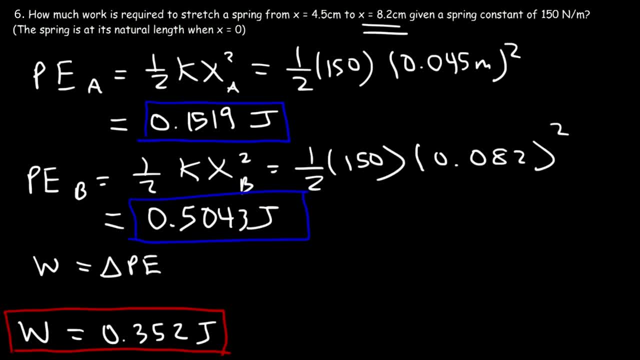 energy. so it's going to be the difference between these two values. so it's point five, zero, four, three minus point one, five from one nine, and so you get the same answer: point three, five, two joules. so the work done by a force is equal to the change in potential energy if the net acceleration. 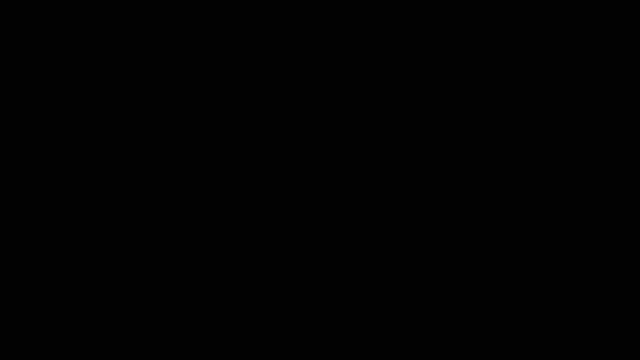 of the system is zero. now there are a few additional details that I want to mention regarding the work required to pull a spring. as I mentioned earlier in the video, FP is the pull-in force, or the force that we use to stretch a spring, and, based on the way the the drawn that we have on a 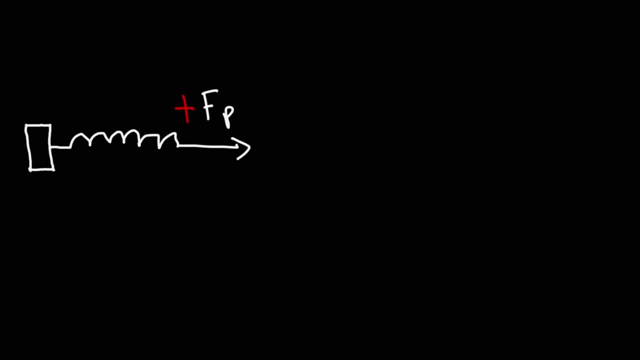 screen, since it's directed to the right. this is going to be defined as a positive force and we described FS as the force exerted by the spring, which is a restoring force. that force tries to bring the spring back to equilibrium. as we stretch the spring to the right, the 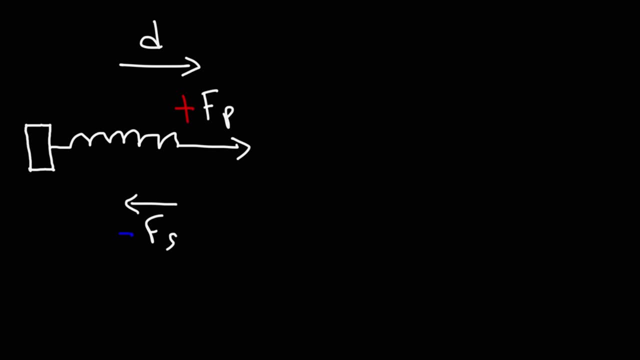 displacement vector is towards the right and we know that work is forced times displacement- notice that these two factors are in the same direction. therefore, the work that's required to stretch a spring is positive. now, the work that's done by the spring itself, as it pulls the spring back to equilibrium, that work is negative. As you can see, the force. 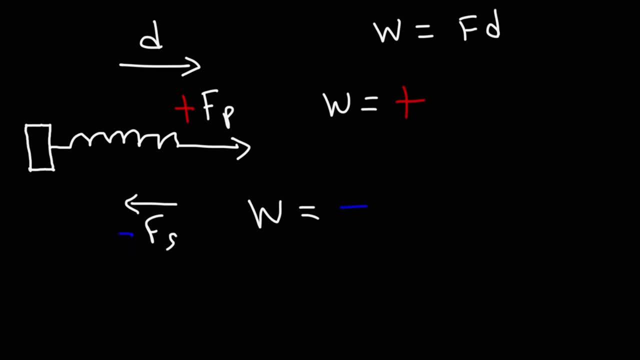 and the displacement vectors. they're in opposite directions. So therefore, the work required to stretch a spring is positive: 1 half k. delta x squared Now, the work done by the elastic force, that is Fs, the work done by the spring, that's. 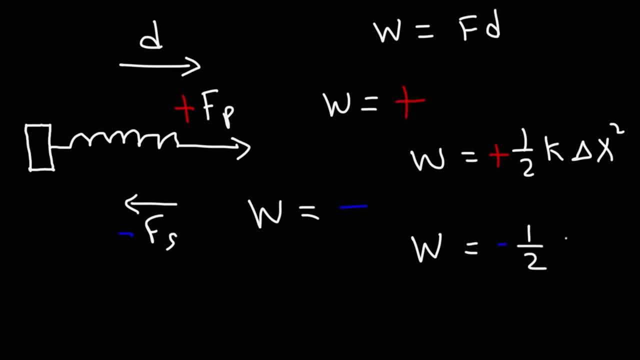 going to be negative: 1 half k delta x squared- as the spring is being pulled to the right Now. the work required to stretch a spring is positive: 1 half k delta x squared Now. this makes sense because in other videos I mentioned that the work done by conservative 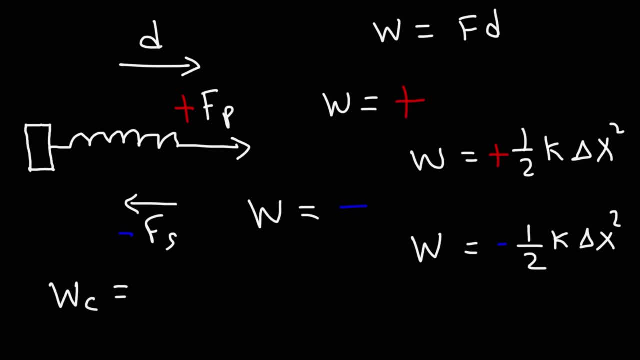 forces like gravity, the electric force or, in this case, the elastic force. negative Fs. that work is negative times the change in potential energy, And the change in potential energy is equal to this expression. It's 1 half k delta x squared.